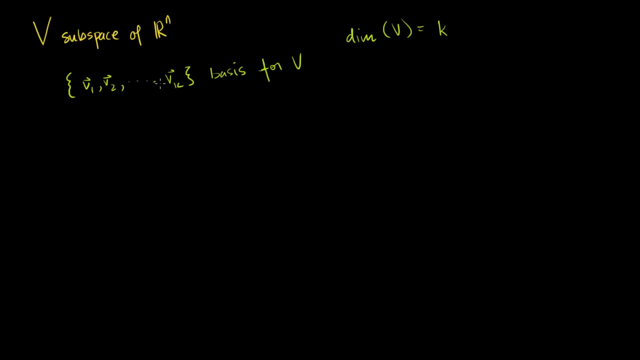 Let's construct a matrix whose column vectors are these basis vectors. So let's construct a matrix A And let's say it looks like this First column is v1, this first basis vector, right there, v2 is the second one, And then you go all the way to vk, like that: 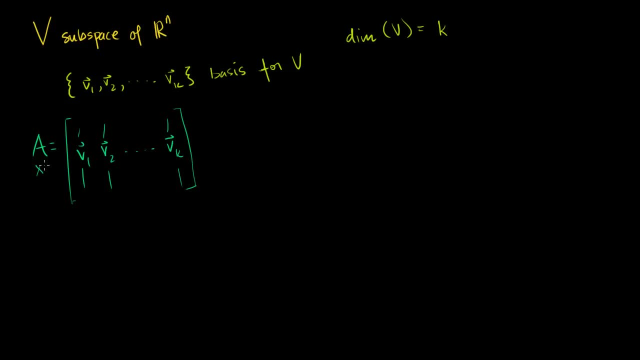 And just to make sure we remember the dimensions, we have k of these vectors, so we're going to have k columns. And then, how many rows are we going to have? Well, there's a member of Rn, so these are all going to have. 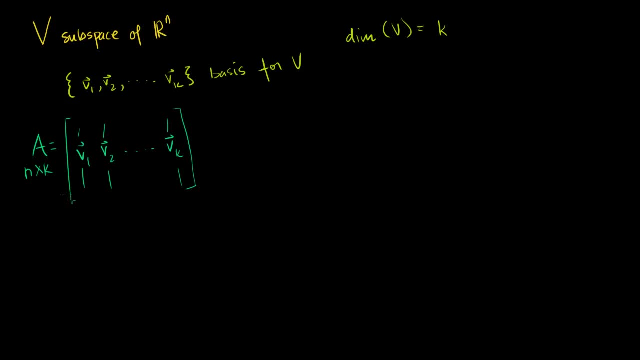 n entries in each of these vectors. So it's going to be an n. We're going to have n rows and k columns. It's an n by k matrix. Now what's another way of expressing the subspace v? Well, we're going to have sub space v. 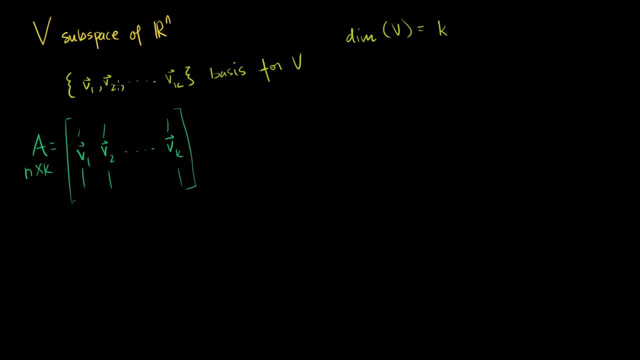 The basis for v is spanned by these basis vectors, which are the columns of these. So if I talk about the span, let me write it this way: v is equal to the span of these guys: v1,, v2,, all the way to vk. 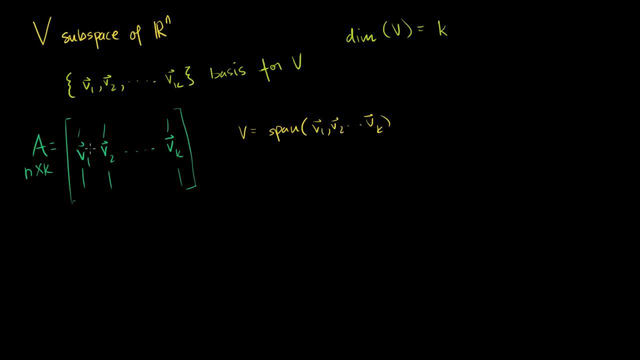 And that's just the same thing as the column space of A. These are the column vectors and the span of them that's equal to the column space of A. Now I said a little while ago we want to somehow relate to the orthogonal complement of v. 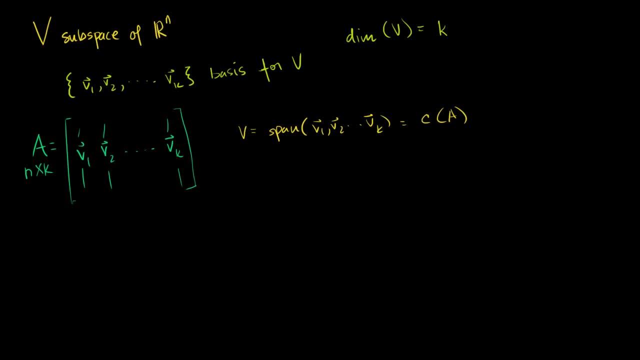 Well, what's the orthogonal complement of the column space of A? The orthogonal complement of the column space of A? I showed you- I think it was two or three videos ago- that the column space of A's orthogonal complement is equal to you. 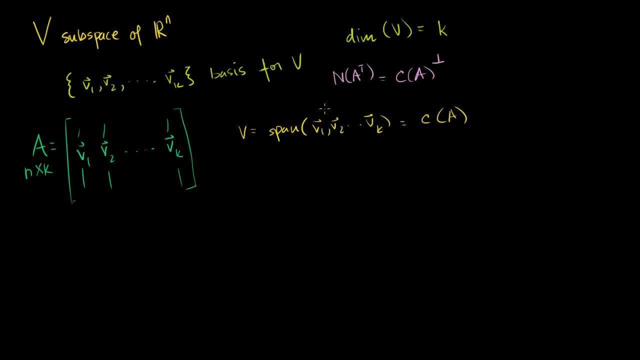 could either view it as the null space of A transpose or another other way you could call it. this is the left null space of A To the orthogonal complement of the column space of A, which is also going to be equal to, which is also since this piece. 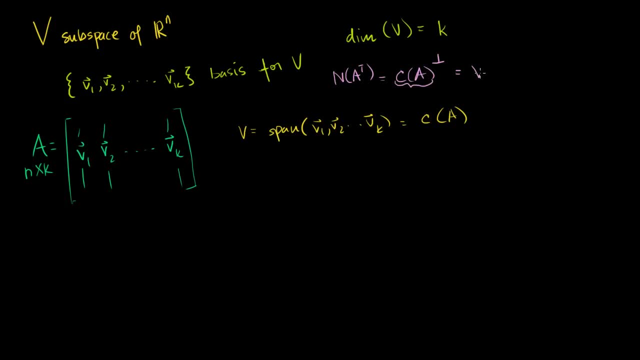 right here is the same thing as v if you take its orthogonal complement. that's the same thing as v's orthogonal complement. So if we want to figure out the dimension of the orthogonal complement of v, we just need to figure out the dimension of. 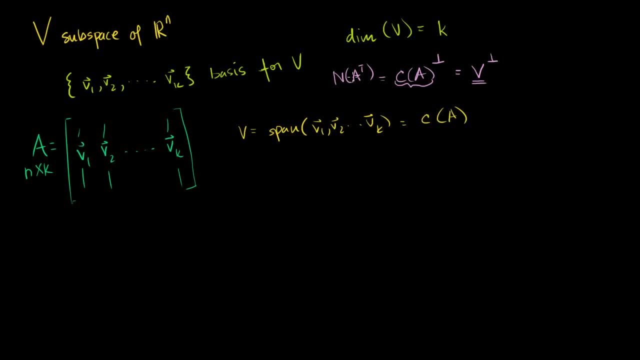 the left null space of A or the null space of A's transpose. Let me write that down. So the dimension- I'm getting you tongue-tied sometimes- The dimension of the orthogonal complement of v is going to be equal to the dimension of A transpose. 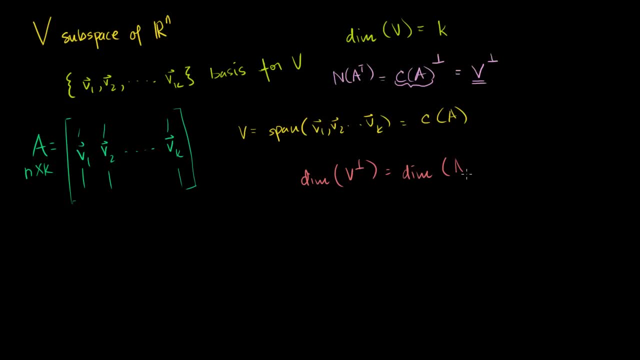 Or another way to think of it is sorry, not just the dimension of A: transpose, the dimension of the null space of A transpose. The dimension of the null space of A transpose- And if you have a good memory, I don't use the word a lot- 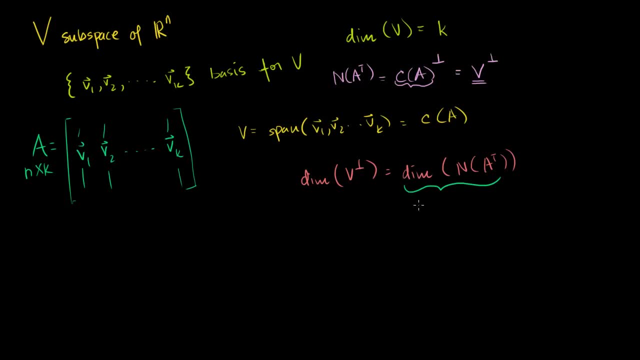 this thing is the nullity. This is the nullity of A transpose. The dimension of your null space is nullity. The dimension of your column space is your rank. Now let's see what we can do here. So let's just take A transpose. 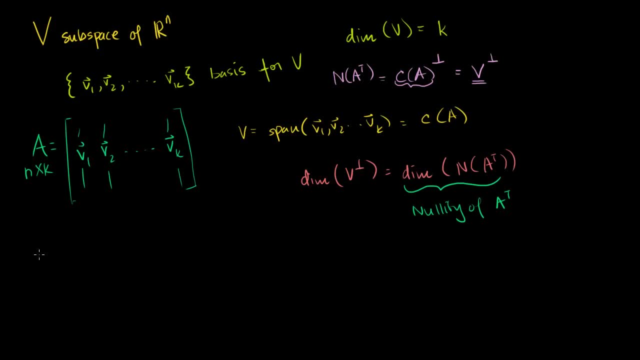 So you could just imagine A transpose for a second. So A transpose, I could just even draw it out. It's going to be a k by n matrix. It's going to be a k by n matrix. that looks like this: These columns are going to turn into rows. 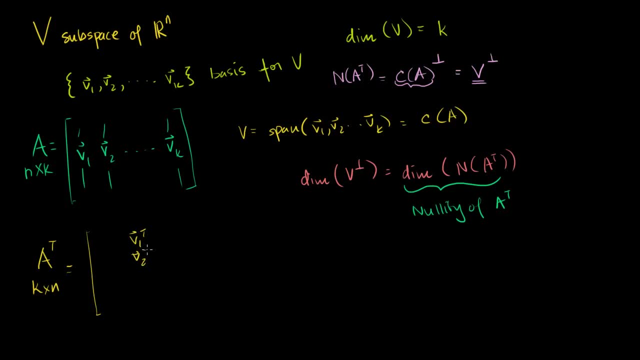 This is going to be v1 transpose, v2 transpose all the way down to vk transpose It's vectors. So these are all now row vectors. So we know one thing. We know one relationship between the rank and nullity of any matrix. 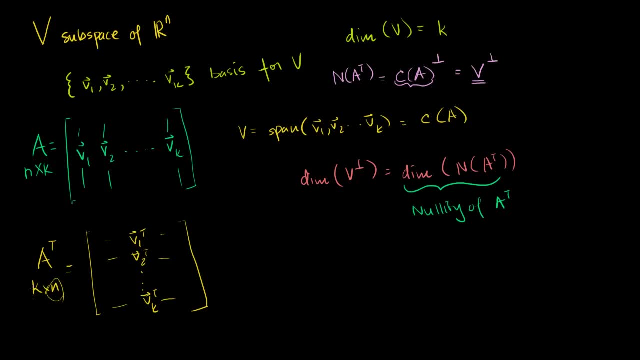 We know that they're equal to The number of columns we have. We know that the rank of A transpose plus the nullity of A transpose is equal to the number of columns of A transpose. So we have n columns. Each of these have n entries. 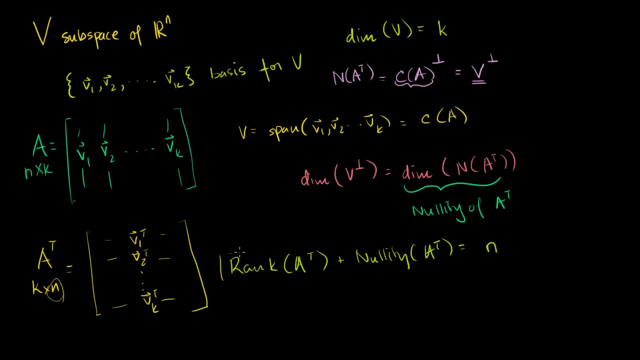 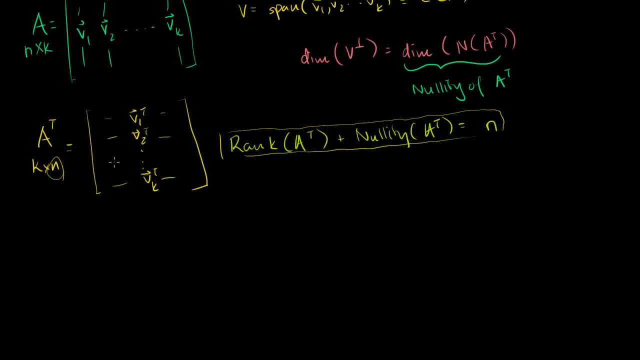 It is equal to n. We saw this a while ago. If you want just a bit of a reminder of where that comes from When you take A, if I wrote A, transpose as a bunch of column vectors which I can, Or maybe let me take some other vector b, because I want to. 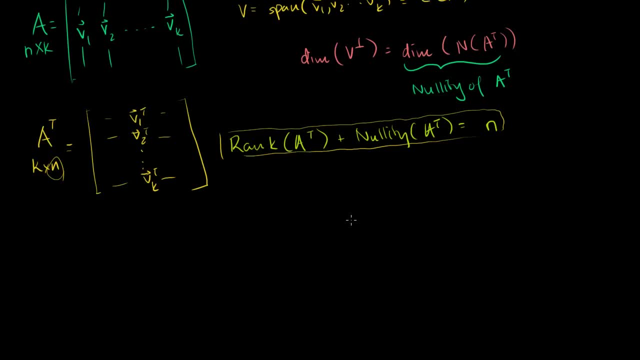 just remind you why this made sense. If I take some vector b here and it's got a bunch of column- vectors- b1, b2, all the way to bn- and I put it into reduced row echelon form, you're going to have some pivot columns and 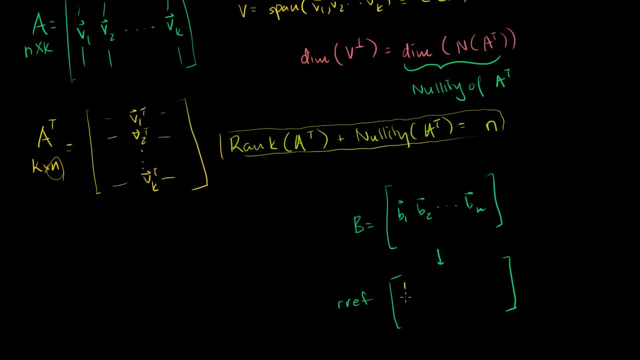 some non-pivot columns. So let's say: this is a pivot column. You know, I've got a 1 and a bunch of 0's. Let's say that this is one of them, And then let's say I've got one other one, that's out. 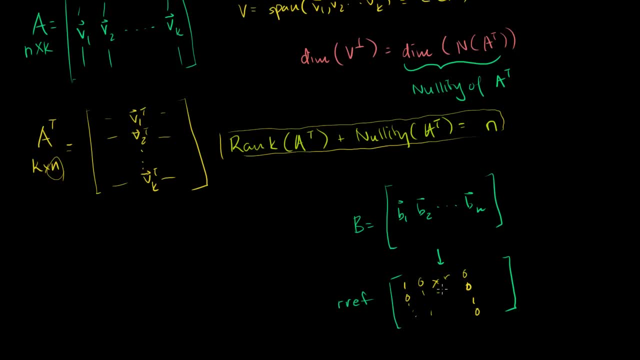 It would be a 0 there. Let's say it's a 1 down there And everything else is a non-pivot column. I showed you in the last video that your basis for your column space is the number of pivot columns you have. 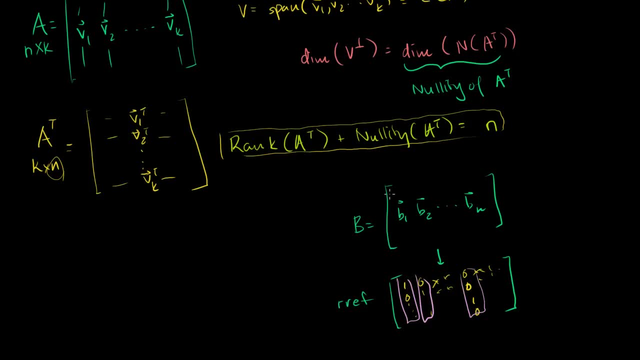 So these guys are pivot columns. The corresponding column vectors form a basis for your column space. I showed you that in the last video, And so if you want to know the dimension of your column space, you just have to count these things. You just count these things. 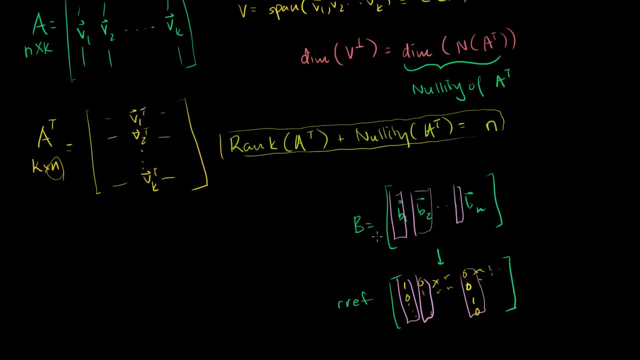 This was equal to the number of. well, for this B's case, the rank of B is just equal to the number of pivot columns I have. Now. the nullity is the dimension of your null space And we've done multiple problems where we found the 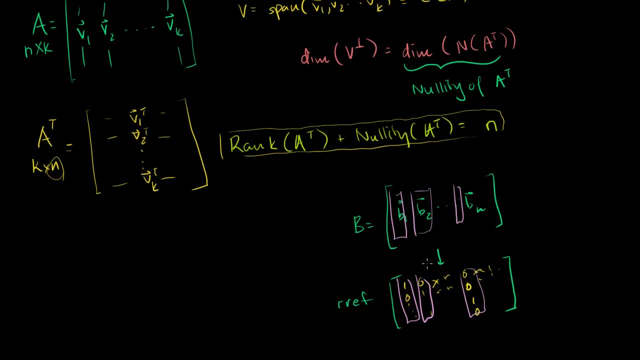 null space of matrices And every time the dimension. it's a bit obvious and I actually showed you this proof- it's related to the number of free columns you have or non-pivot columns. So if you have no pivot columns, then if you have no. 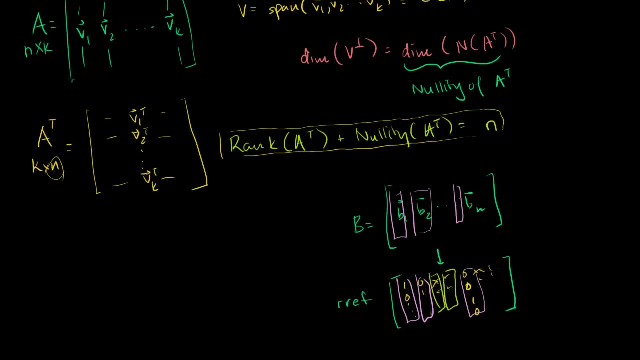 pivot columns. if all of your columns are pivot columns and none of them have free variables or are associated with free variables, then your null space is going to be trivial. it's just going to have the 0 vector. But the more free variables you have, the more 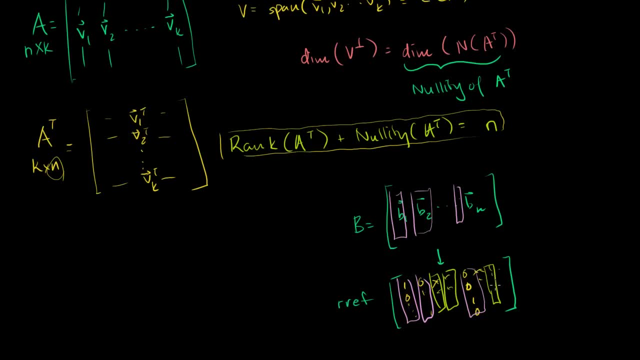 dimensionality your null space has. So the free columns correspond to the null space and they form actually a basis for your null space And because of that the basis for your null space- vectors plus the basis for your column space- is equal to the total. 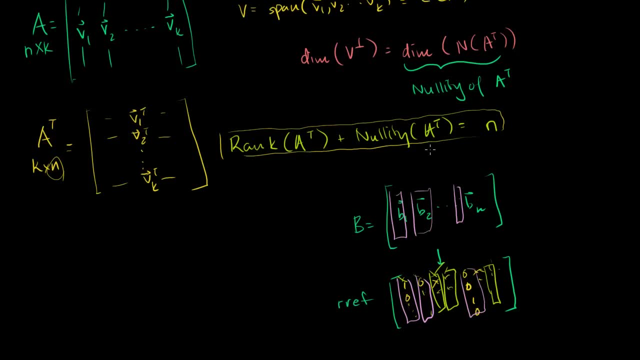 number of columns you have. I showed you that, to you in the past, but it's always good to remind ourselves where things come from. But this was just a bit of an aside. I did this with a separate vector b just to remind.